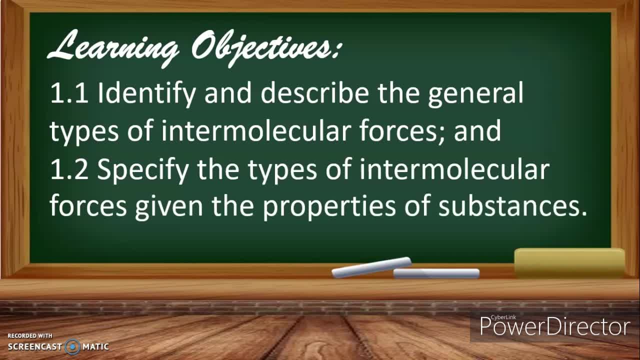 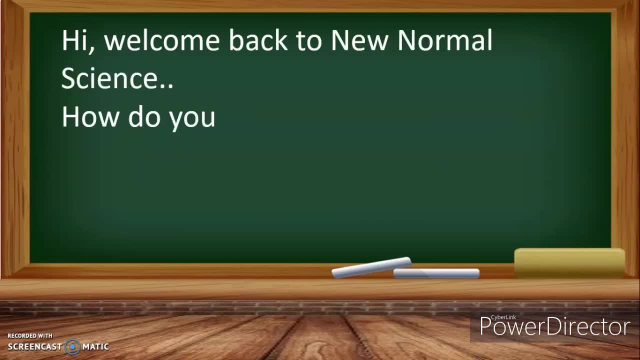 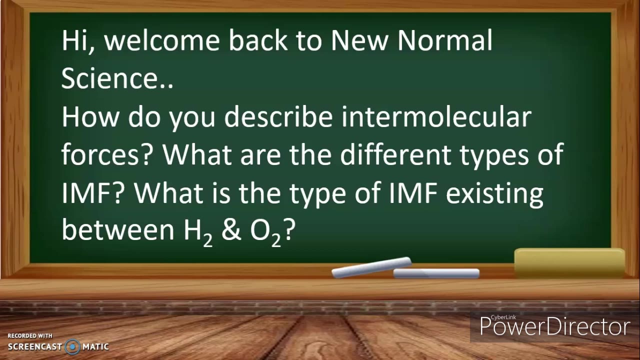 and specify the types of intermolecular forces, given the properties of substances. Welcome back to the new normal science. How do you describe intermolecular forces? What are the different types of intermolecular forces? What is the type of intermolecular force existing between hydrogen and oxygen? 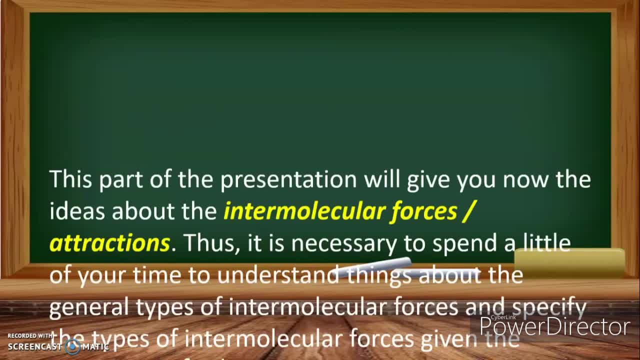 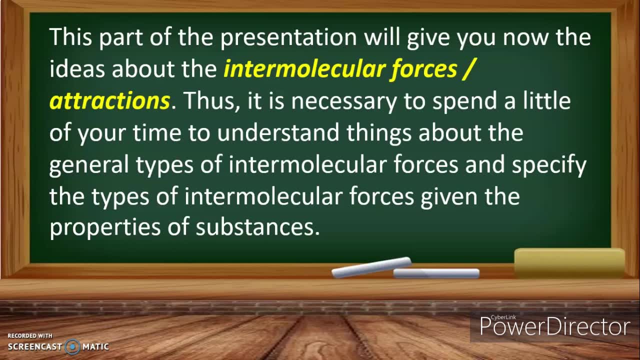 So these are the questions that we are going to answer. This part of the presentation will give you now the ideas about the intermolecular forces of attractions. Thus, it is necessary to spend a little of your time. Thank you for watching. See you in the next video. 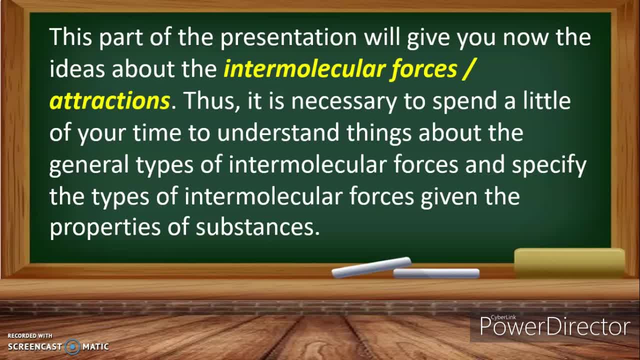 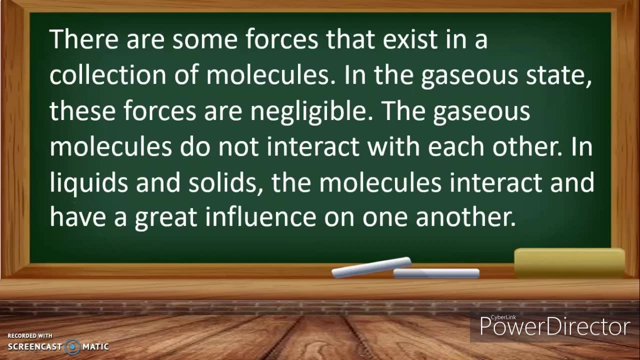 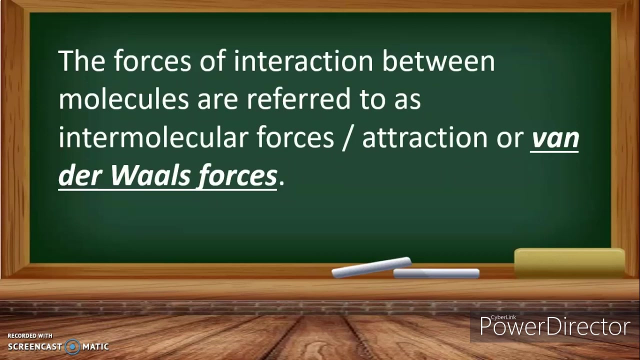 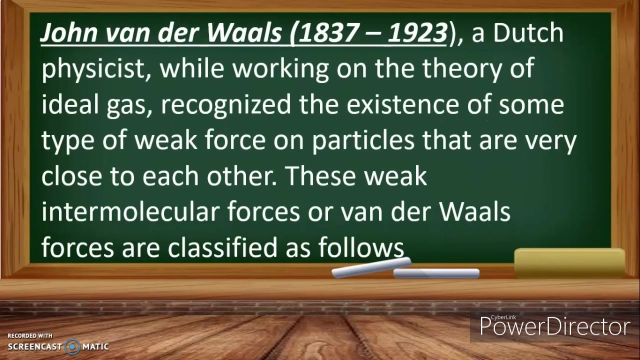 Bye. Thank you for watching, Bye. See you in the next video, Bye, Bye. Subscribe to our channel for personal instructions related to international trazer science. Until then, good luck, Bye, Take care, Bye, Bye, Bye. 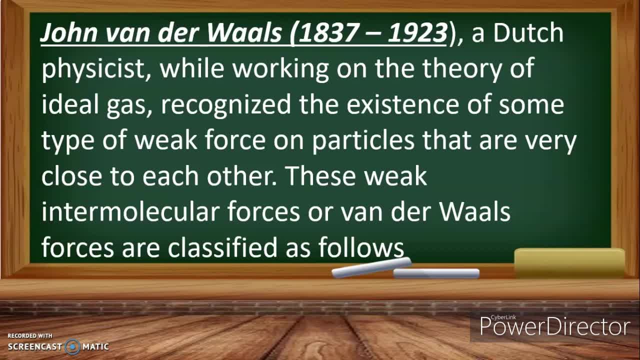 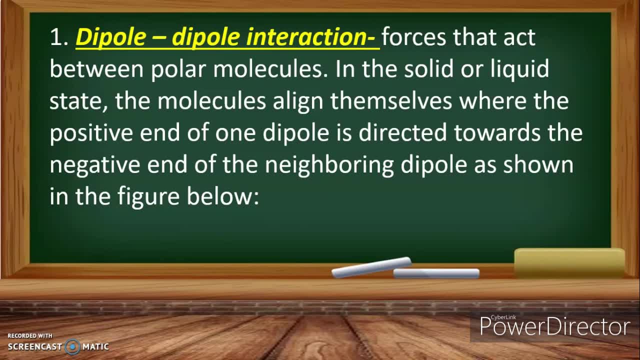 Bye, Bye, Bye walls. forces are classified as follows: dipole-dipole interaction- forces of act between polar molecules in the solid or liquid state. the molecules align themselves where the positive end of one dipole is directed towards the negative end of the neighboring dipole, as shown in the figure below. as you remember in 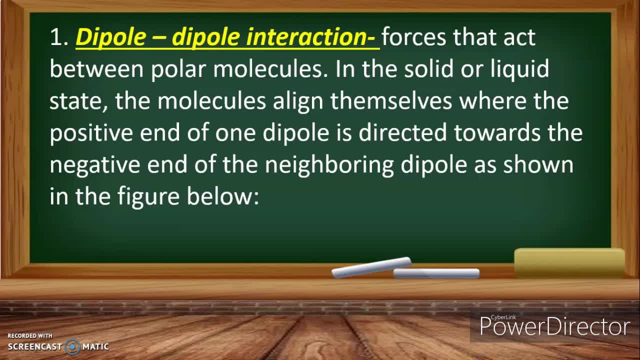 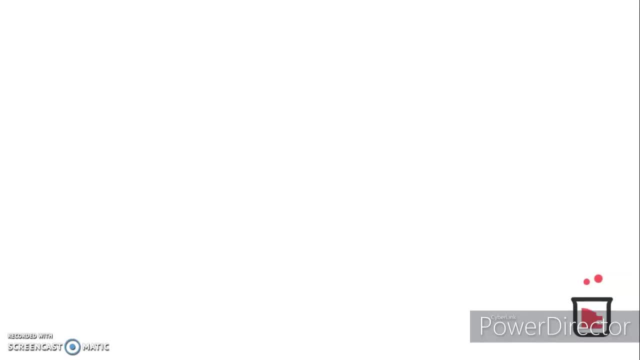 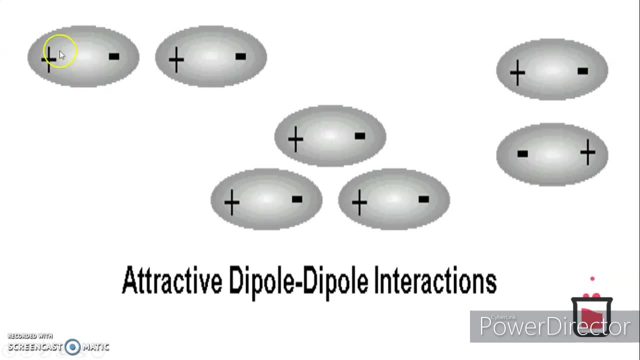 our lesson 1, it is explained that intermolecular is the attraction between poles or charges. so this is an attractive dipole-dipole interaction. as you can see, it shows the ends of their poles. we have positive and negative. then the negative is attracted to positive, negative attracted to positive. 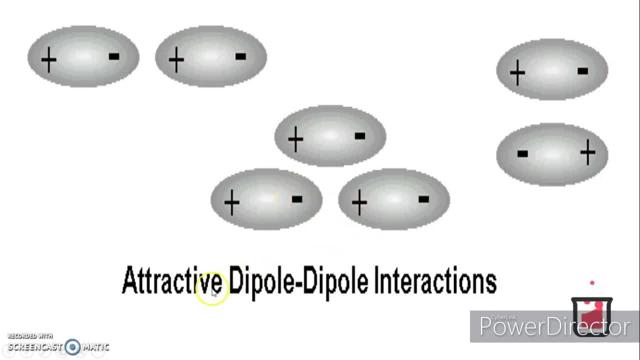 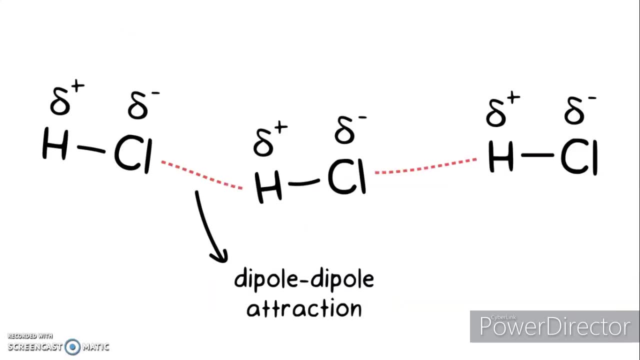 attracted to negative. so that is their attractive dipole-dipole interaction. a very good example of this one is hydrogen chloride or hydrochloric acid. so that is the dipole-dipole attraction between the molecules of hydrogen chloride. so we have the negative charge n of chloride and the positive 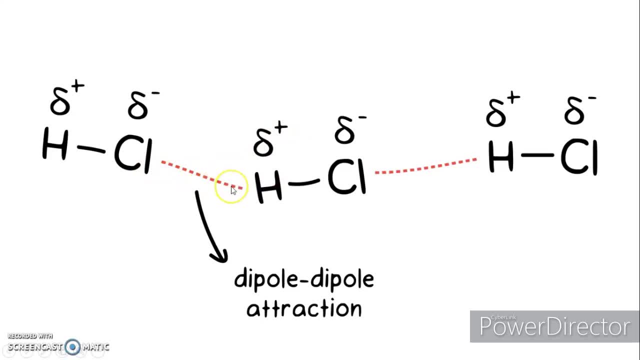 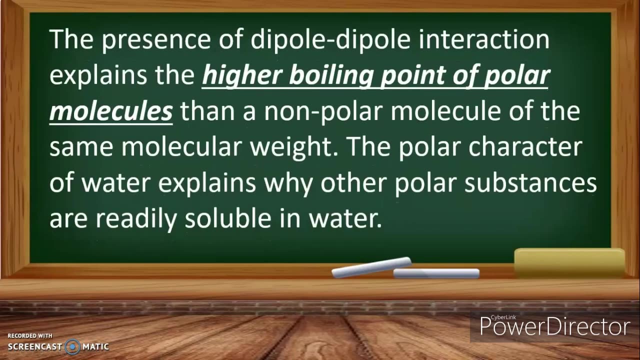 n of hydrogen. so they are attracted with one another, so they are interconnected by this type of force, the dipole-dipole attraction. the presence of dipole-dipole interaction explains the higher boiling point of the polar molecules than a nonpolar molecule of the same molecular weight. 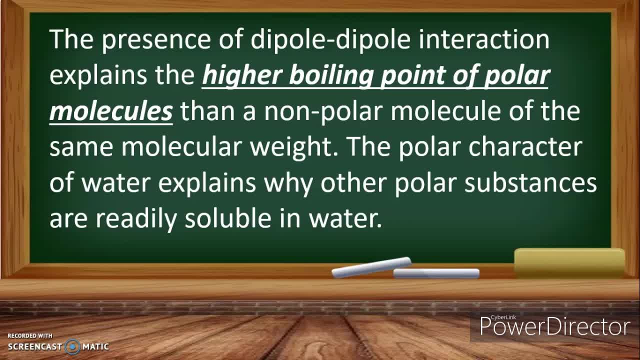 the polar character of water explains why other polar substances are readily soluble in water. so remember in the last class we have mentioned that the polar- our lesson in chemistry- we have likes, dissolves likes. if a polar molecule or substance is put or placed in water, that is uh, which is soluble. it will become soluble in water. hydrogen bonding. 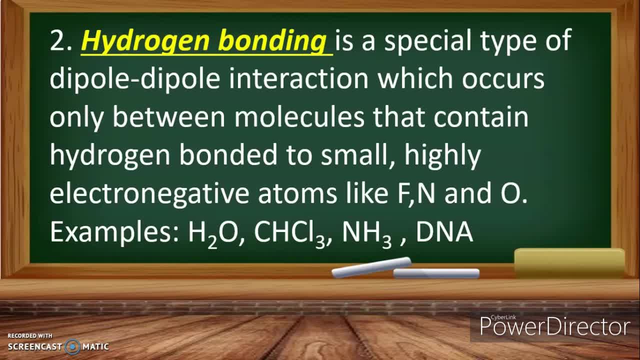 is a special type of dipole-dipole interaction, which occurs only between molecules that contain hydrogen bonded to small highly electronegative atoms like fluorine, nitrogen and oxygen. examples: we have h2o or water, we have chcl3 or chloroform, we have 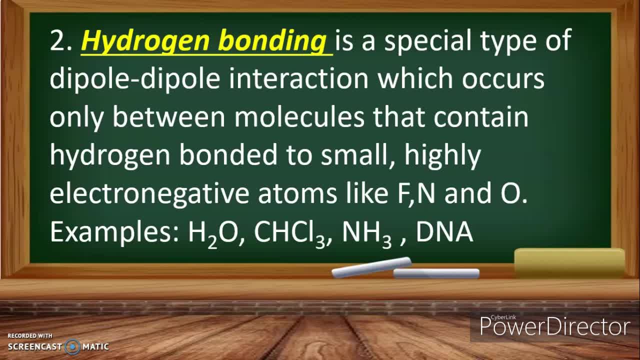 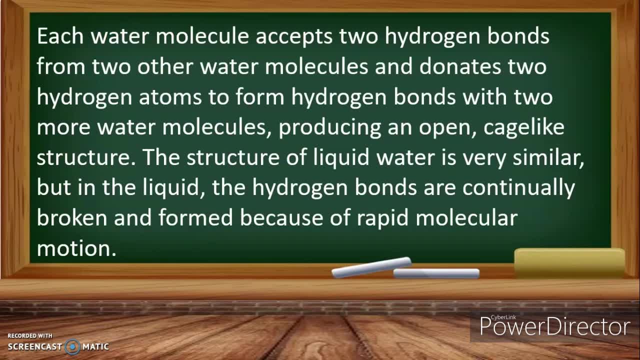 nh3 or ammonium, and we have dna or deoxyribonucleic acid. each water molecule accepts two hydrogen bonds from other water molecules and donates two hydrogen atoms to form hydrogen bonds with two more water molecules, producing an open cage-like structure. so the structure of liquid. 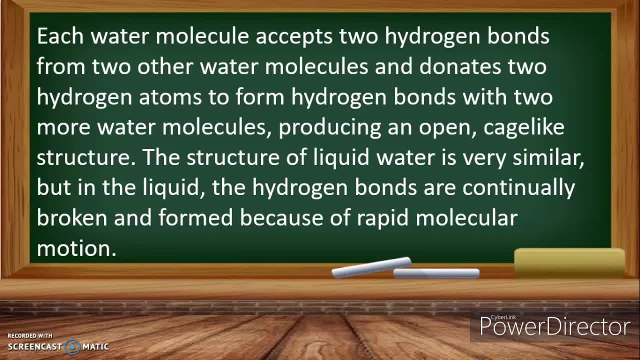 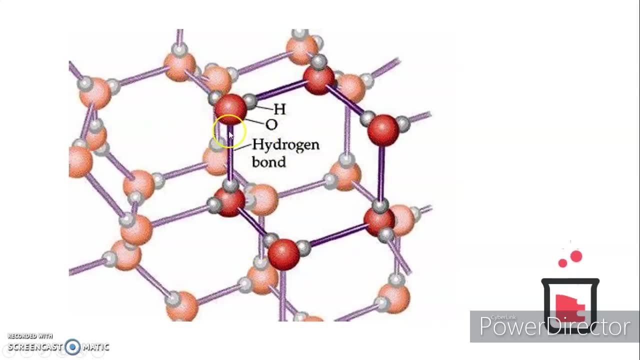 water is very similar, but in the liquid the hydrogen bonds are continually broken and form because of rapid molecular motion. so let's take a closer look of the structure. so this is the structure of water molecule. so, as you can see, it's like a close, cage-like structure. 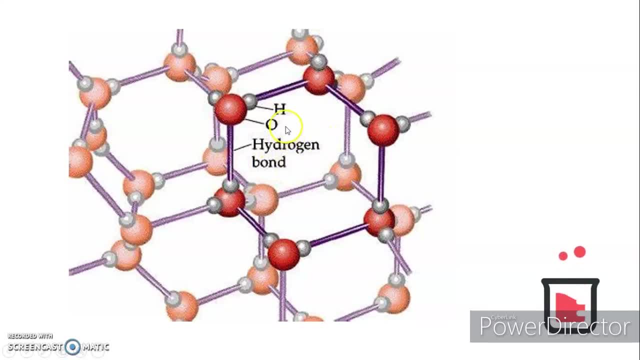 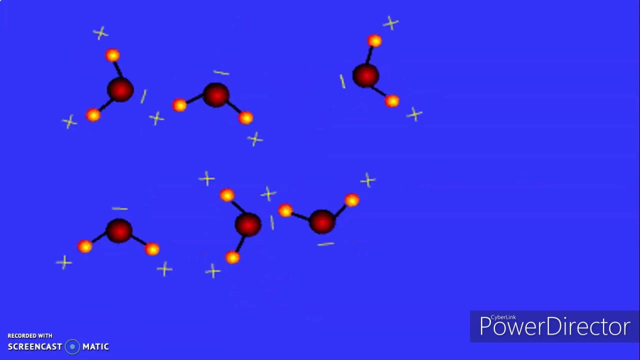 because of the charges or ends of the hydrogen and oxygen and they are bonded together by a hydrogen bond. hydrogen bond is not a strong bond compared to the other types of intermolecular forces there. as you can see, it shows the positive and negative charges and the type of bond that. 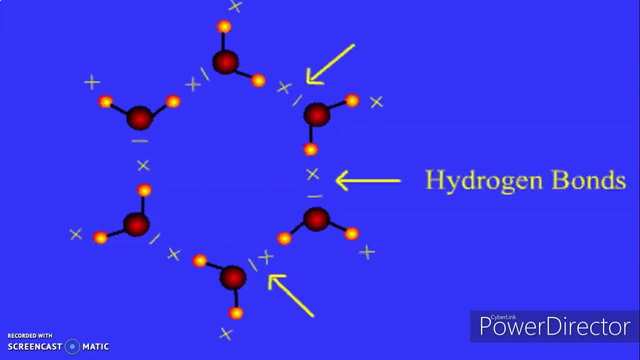 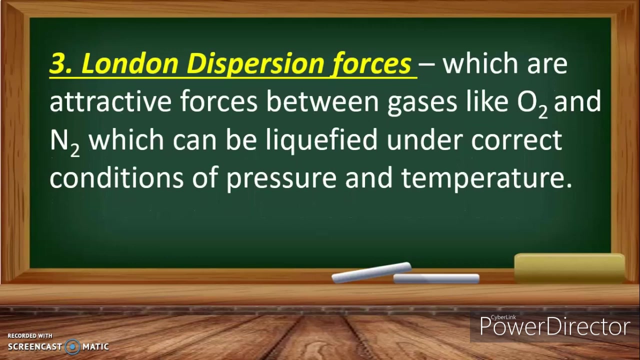 occurs when you convert two particles of water between a spline into an intermolecular. so you can see theREW has many different types of hydrocarbons, but hydrogen bonds其實 are also energy caused by a strong bond, and this is the main reason why hydrogen bonds remain green. 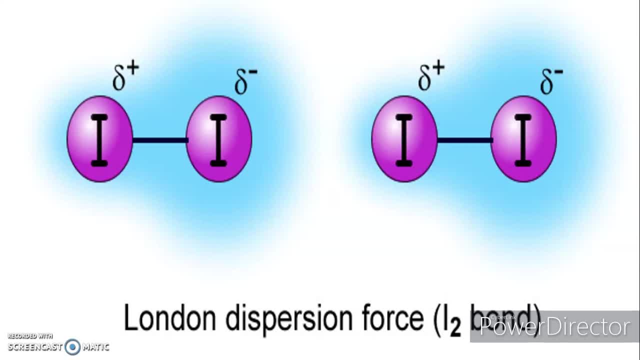 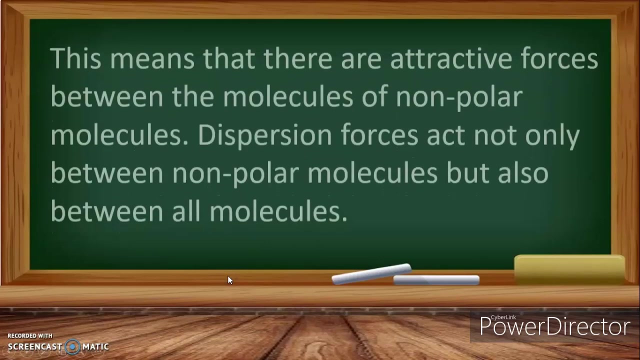 of a London dispersion forces between iodine. so, as you can see, there is a partial charge of positive and a partial charge of negative between iodine atom. so iodine is diatomic, as you can see, and those of the other halogen atoms they are diatomic. this means that there are attractive 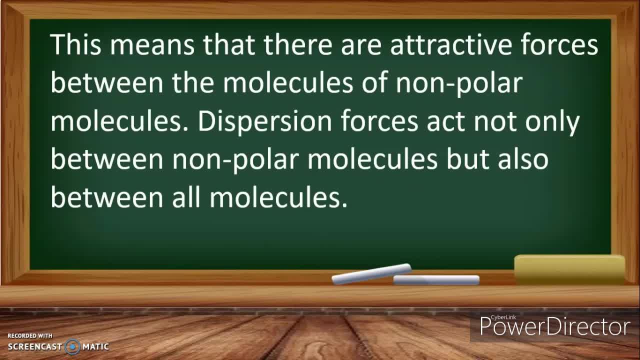 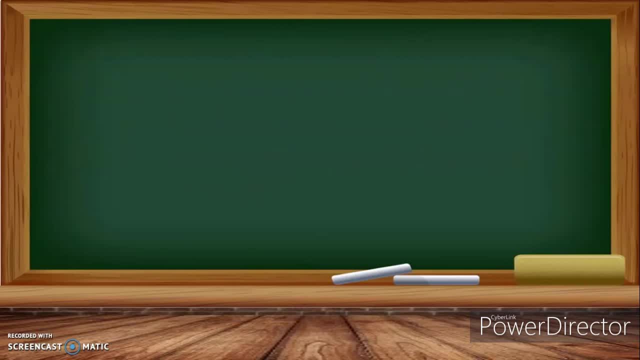 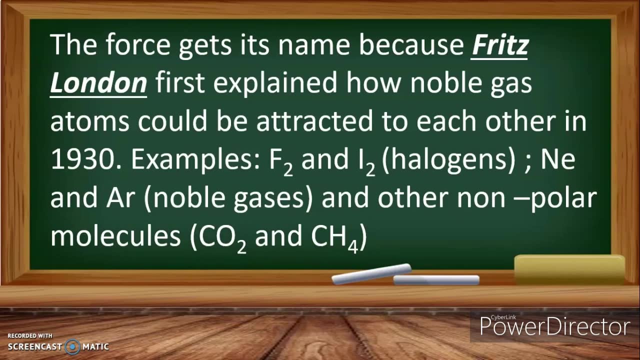 forces between the molecules of nonpolar molecules. dispersion forces act not only between nonpolar molecules but also between all molecules. the force gets name because of Fritz London first explained how noble gas atoms could be attracted to each other in 1930. examples we have fluorine and iodine. so these are 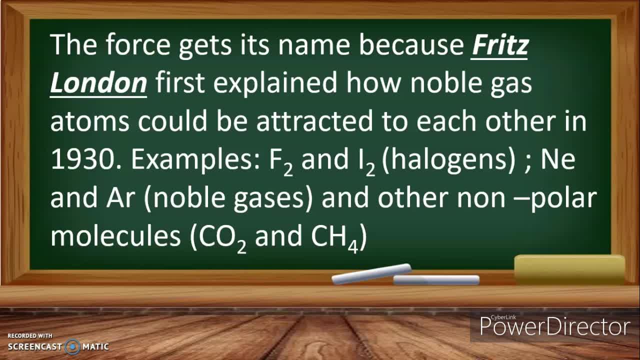 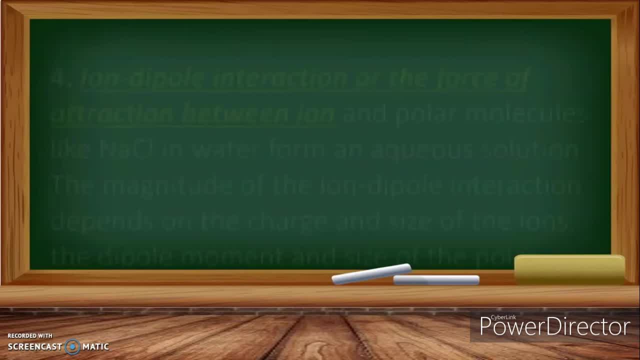 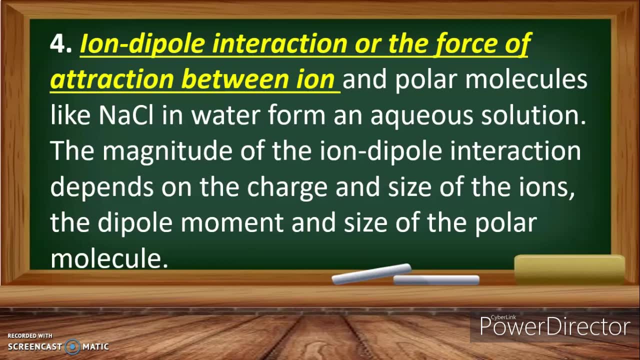 examples of halogens we have neon and argon. these are examples of noble gases and other nonpolar molecules like carbon dioxide and methane. ion-dipole interaction or the force of attraction between ion and polar molecules like sodium chloride in water form, an aqueous solution. so the magnitude of the ion. 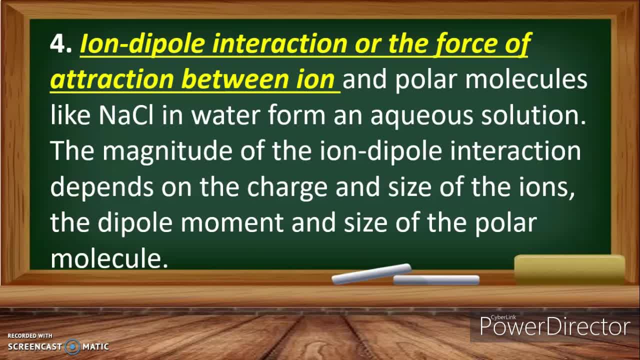 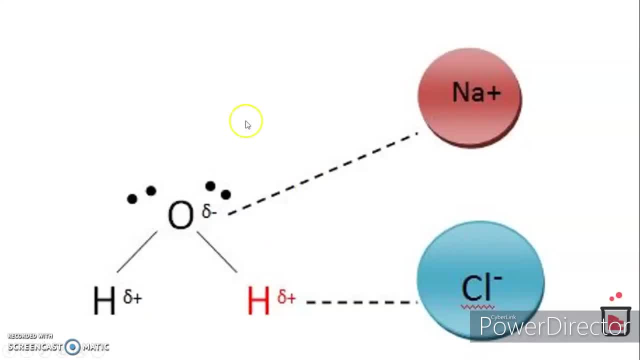 dipole interaction depends on the charge and size of the ions, so the dipole moment and size of the polar molecule. so, as you can see, we have the sodium chloride molecule dissolve in water. as sodium chloride dissociates in water, it forms ions. we have sodium ion and 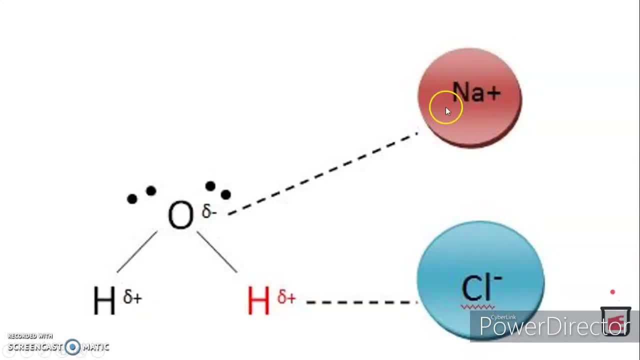 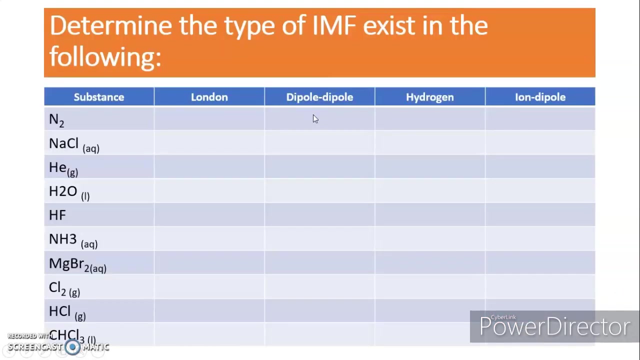 chloride ion. the sodium ion is a cation or positive charge, so it's attracted to the partial negative charge of oxygen, while the chloride ion, which is negatively charged or an ion, is attracted to the partial positive charge of hydrogen. so together they form an ion-dipole force or interaction. now let us 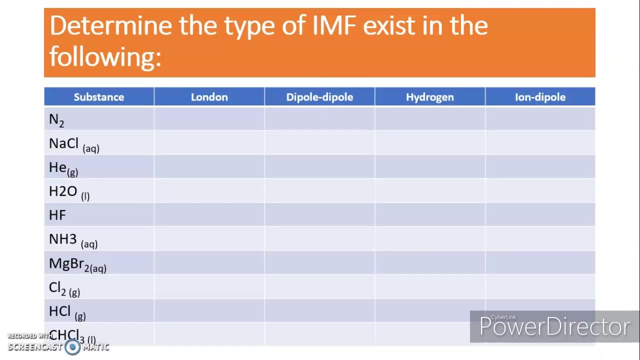 determine the worksheet a while ago. I think you are ready to answer it. let us identify the different substances and their corresponding intermolecular forces. so we have nitrogen. can you guess or answer what is the typhoon life of the intermolecular forces? very good, it's London forces. next one we have 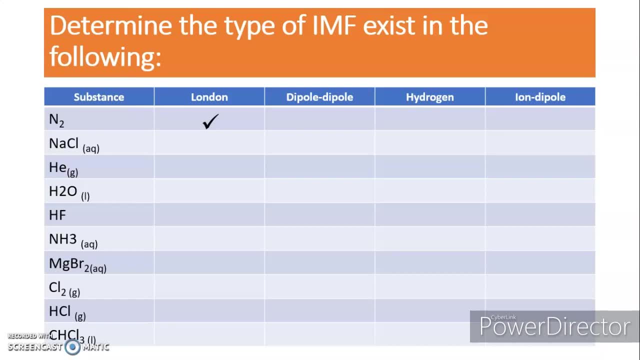 aqueous sodium chloride: very good, its ion dipole. what about Helium gas? very good, its London forces. what about H 2 Oh or water? very good, its hydrogen bond ability. very good, its hydrogen bond ability. very good, its hydrogen bond. how about hydrogen fluoride? yes, it's hydrogen bonding. what about NH3 or aqueous ammonia? very 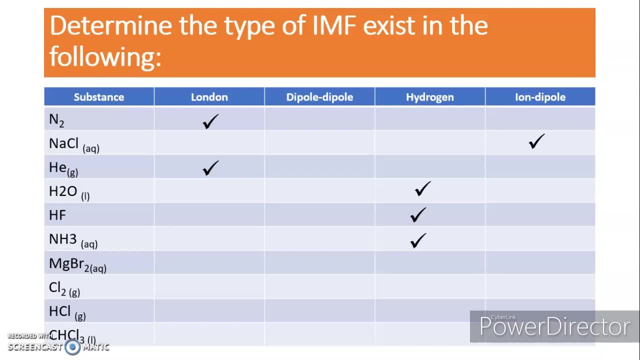 good, it's hydrogen bonding. what about magnesium bromide? yes, it's ion dipole, because magnesium bromide is ionic and when it is dissolved in water it will become magnesium bromide or aqueous magnesium bromide. so it will be dissociate in water, it forms positive for the magnesium and